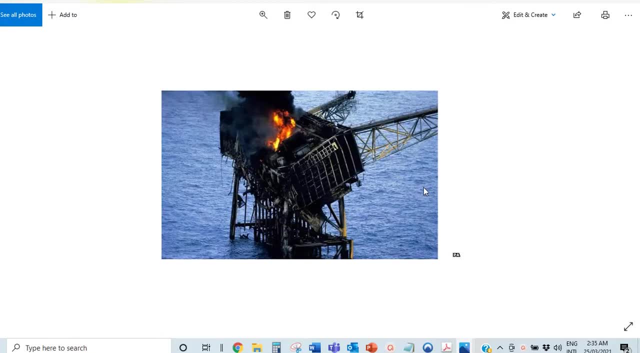 by doing what they were told not to do, which was jump into the water, and this was in the north sea, so you can imagine how cold it was. they had to jump off the platform and into the water. that's how they survived. most of the people that stayed on the on the facility died, and about 30 bodies 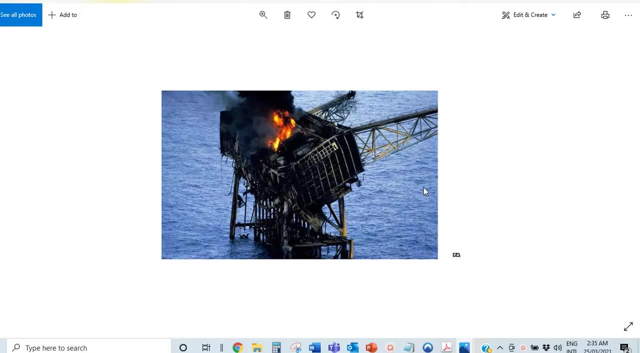 were never, ever recovered and it was. the total loss incurred in monetary figures was about almost two billion dollars, well over a billion, well over 1.5, between 1.5 and 2 billion dollars. that was the loss and it's one of the costliest. 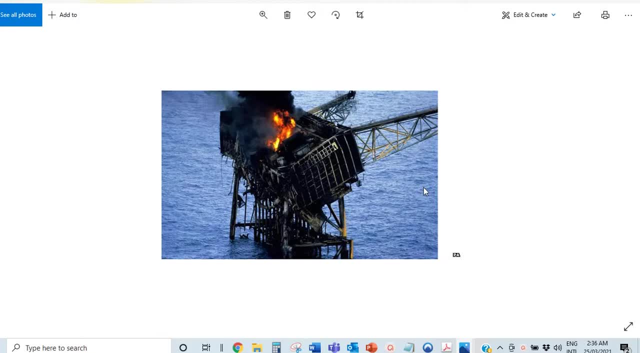 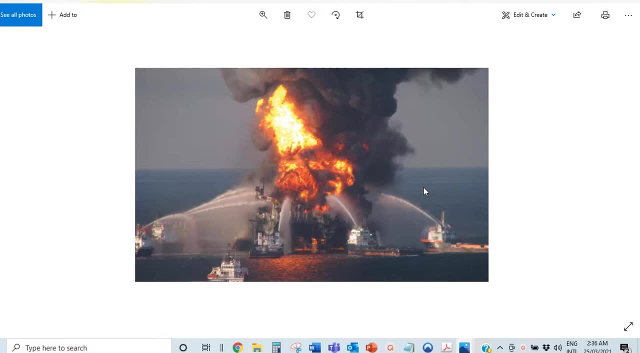 costliest, like accidents ever. it took three weeks for this fire to be extinguished, and so it was. it all started from like a condensate pump. there were two condensate pumps. one was under eps, the other was was working. the guys that were repairing one had removed the. 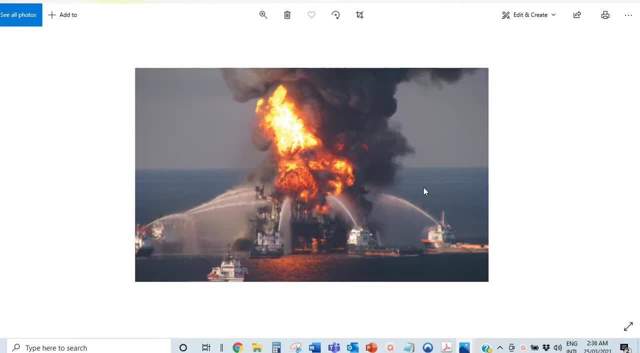 relief valve and they they closed their shift and another set came on and probably they didn't know the other pump was the. the one pump was being repaired so, as that pump was, they're not working. the pump that was presently running actually tripped and failed, so they had to go back to 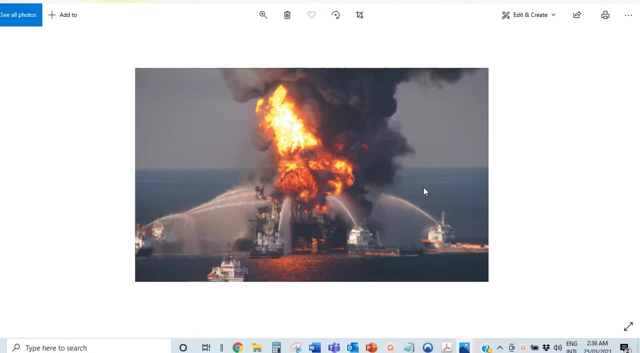 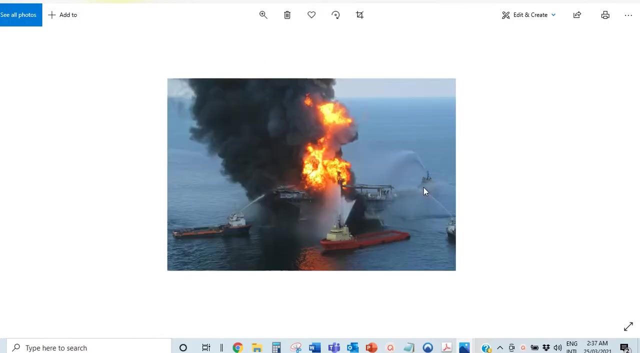 the pump that was under repairs. but they didn't know it was under repairs and the relief valve was off and they tried turning it on or something close to that, and then the fire started. so it was very, very nasty. so that's um, that's Piper Alpha, and this was kind of what led to the modern day process safety, although 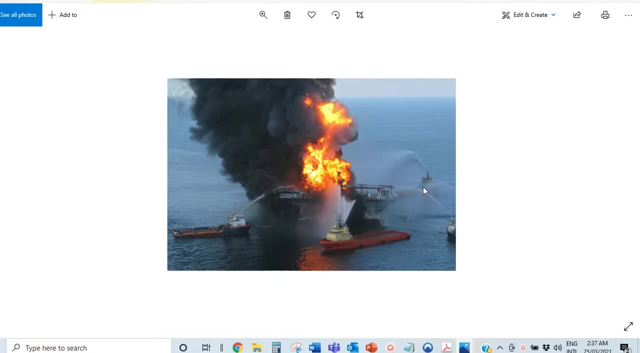 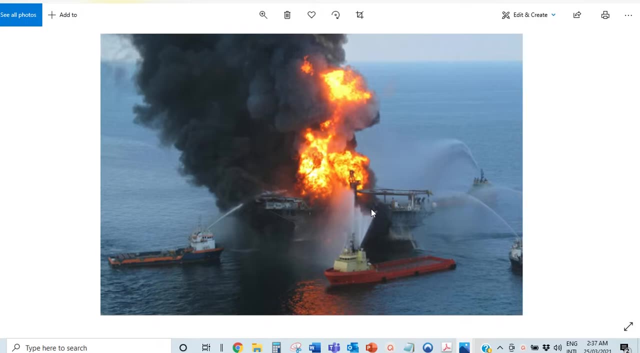 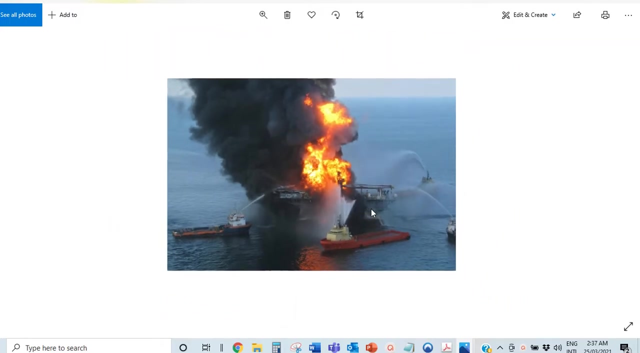 there was safety kind of processing, but modern day times this is kind of what led to it. this accident is has been reviewed, reviewed it in school and i was um doing my masters in Sheffield. we did a lot of work on it and it is a lot of information about it if you just run a google. 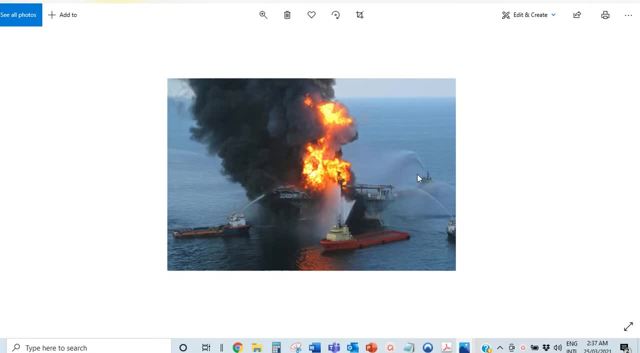 search: Piper Alpha fire, explosion and stuff. so that's what now is the work we've done on my Scбу Day Station of Piper Alpha fire, Master Scboom at Sheffield. we did a lot of work on it and there's a lot of information about it if you just run a Google search: Piper Alpha fire, explosion and stuff. so that's. 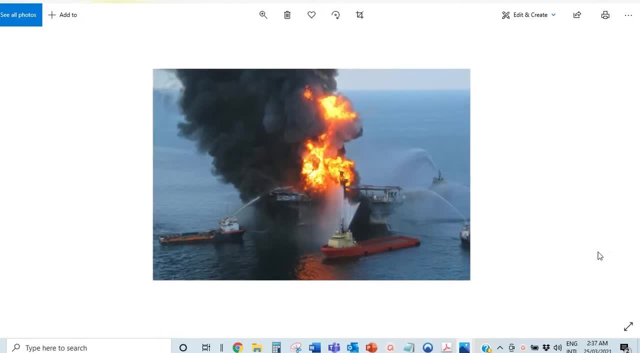 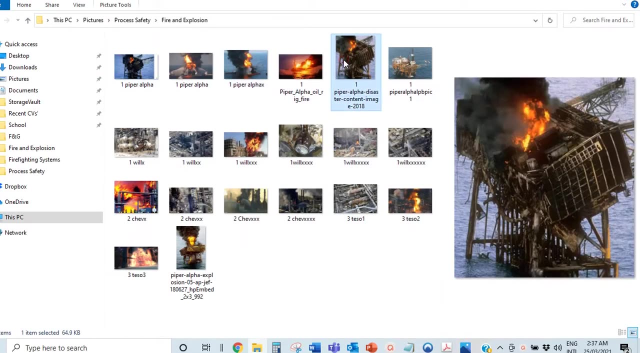 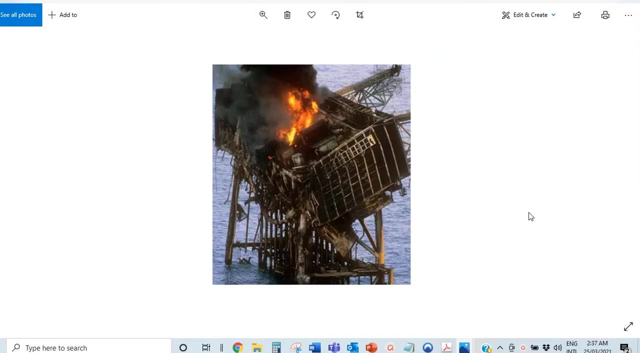 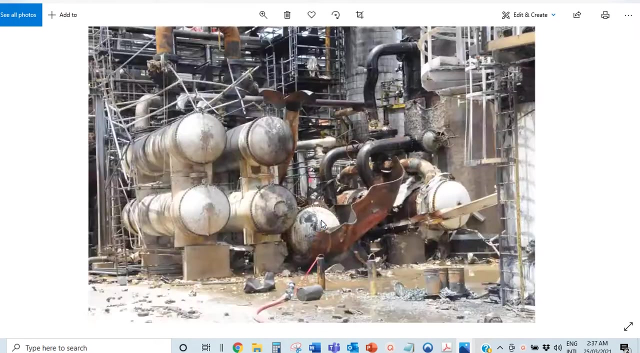 what this is about, then. what's okay then? okay, I showed you how it's kind of ended up being. this is it when you started and this was it at the end, and it just had to be. it was abandoned in the sea and brought down, so next I want to talk. 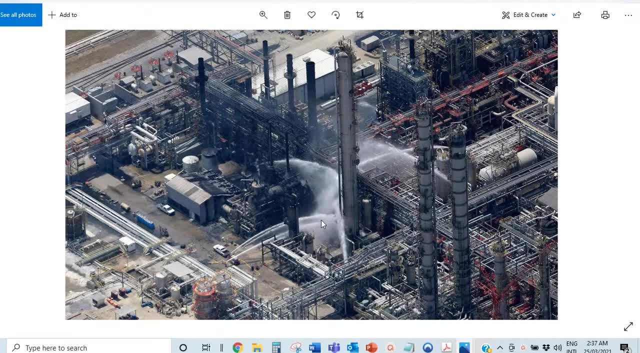 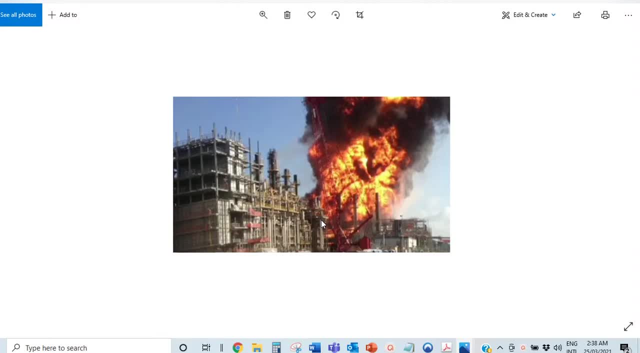 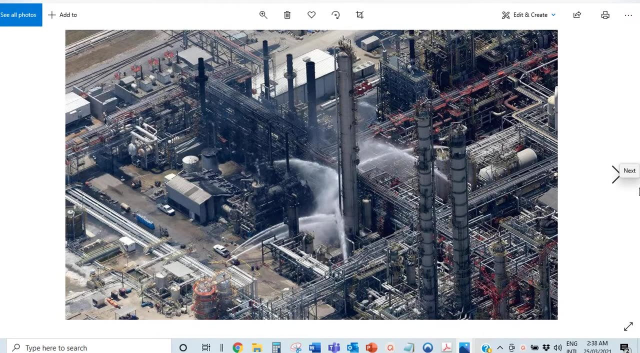 about another. I'm still gonna explain what process safety is, but I want to talk about another plant fire, and this was the Williams plants in Louisiana. this happened in 2018- this does just three years ago- and the explosion was caused by failure of a heat exchanger and two workers died, 114 were injured. this there. 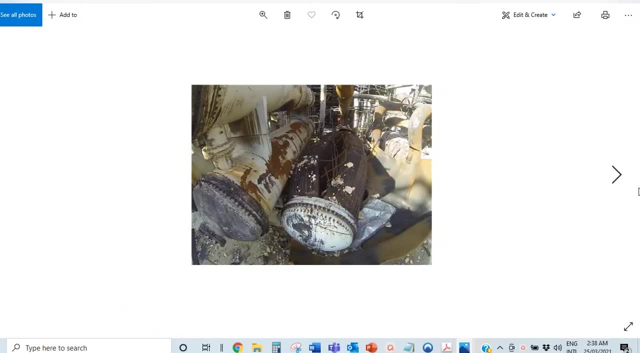 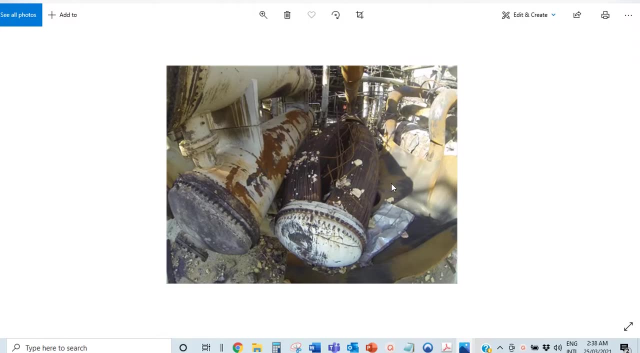 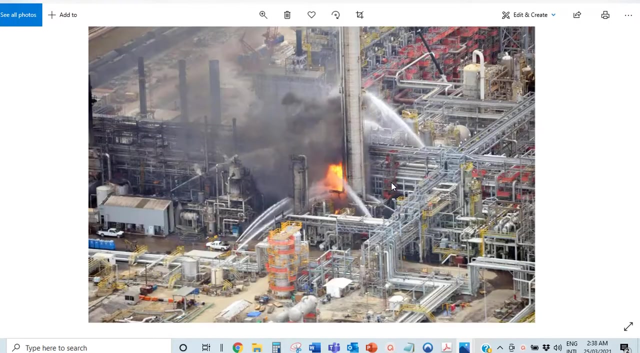 was a rupture in, if you look further down, this, I believe, was the heat exchanger that got ruptured and there were leaks and there was a vapor cloud that was that's flammable vapor cloud which ignited and, yeah, there was a fire and yeah, that's what we had. we had this, this very, very nasty fire. 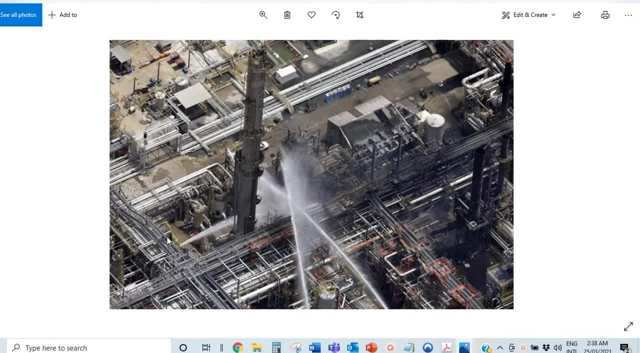 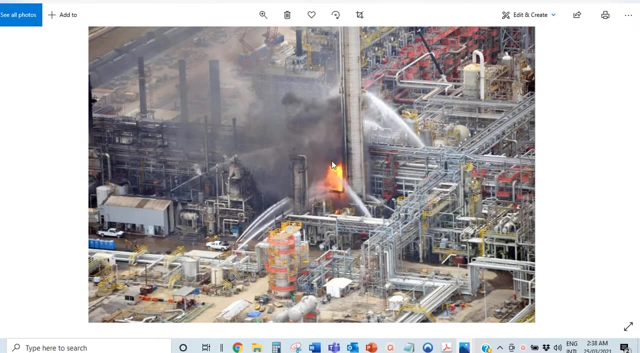 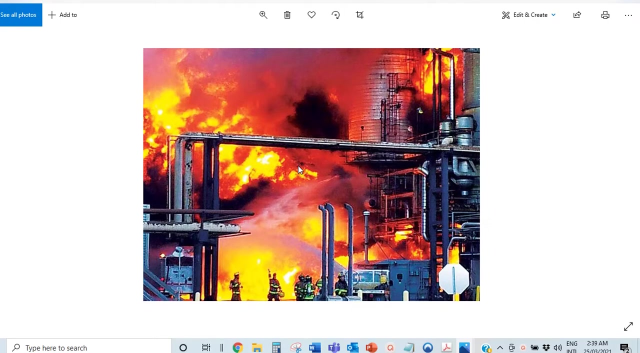 and this was just three years ago- and you can see fire fighting. you can see a lot of water probably coming from maybe hydra monitors, fire water monitors and fire trucks trying to put out the fire. then I also want us to look at. there was also the Chevron fire, in which 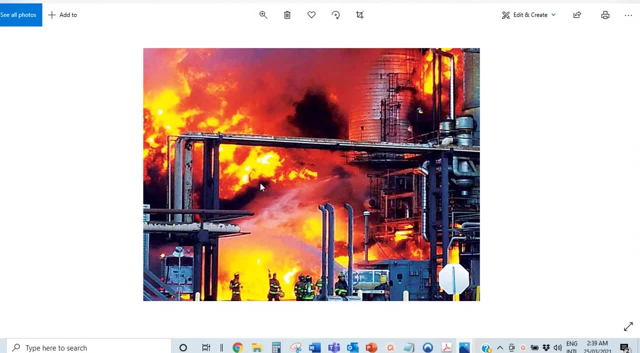 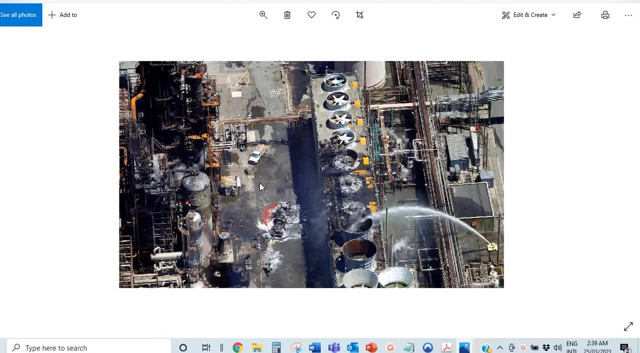 happened in California in 2012. this facility used to process over two hundred and fifty thousand barrels of gas- that's petrol and diesel- every day, and this fire was a nasty one over. I'm not sure if people died- I don't think anyone really died- but over 15,000 people had to go for treatment because 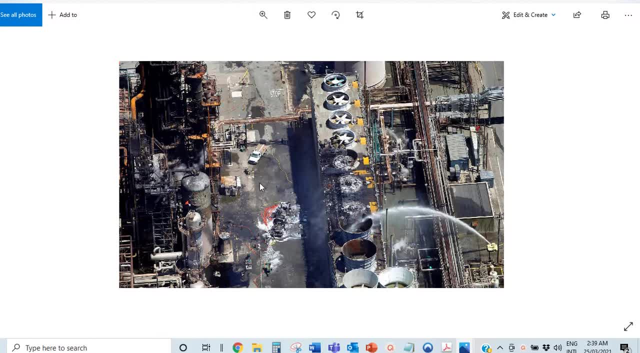 of respiratory disorders. it started from a diesel leak in in a line and the fire. I don't know the full story, but the fire erupted and the diesel- the diesel fires- always born with a lot of tick-tock smoke, which was what affected a lot of people. some people had some burns on during the fire, so that was. also. 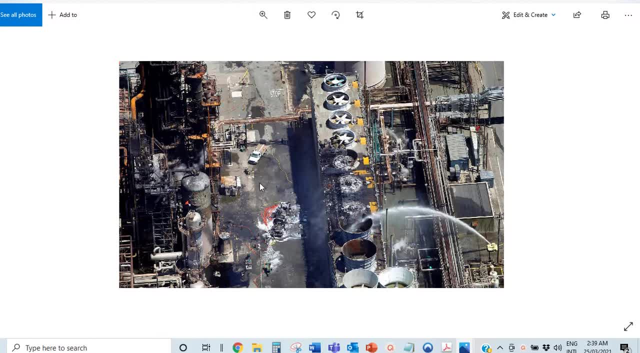 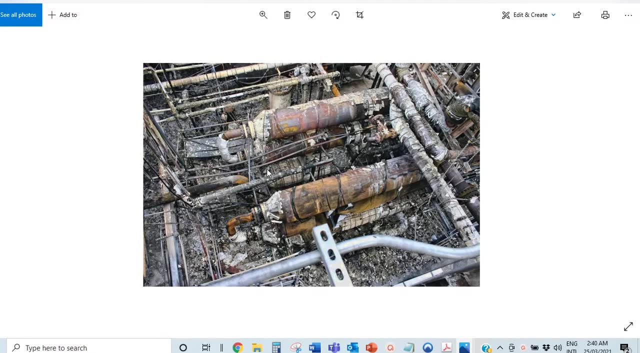 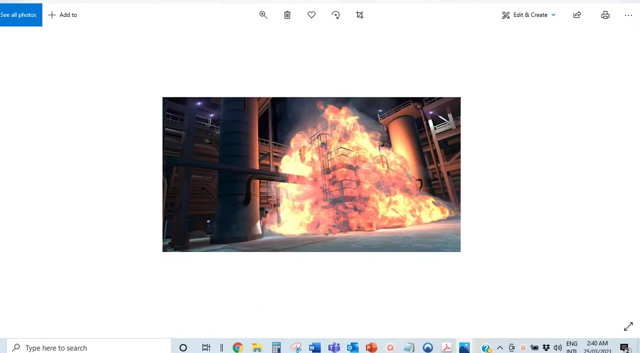 another issue and then what's the last one? okay, this is. this is now Tercero. Tercero refinery explosion. this is in Washington, Washington in the US, and explosion that led to about seven employees dying. really nasty stuff. this was an old heat exchanger that failed. 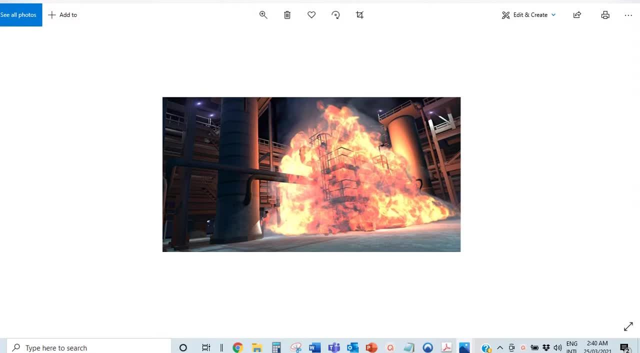 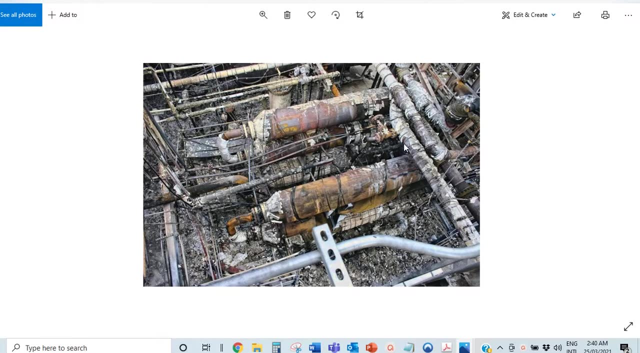 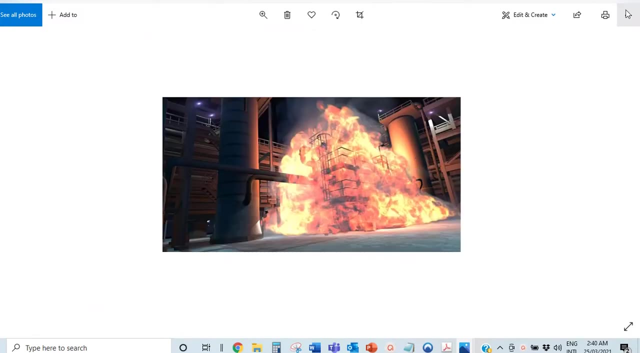 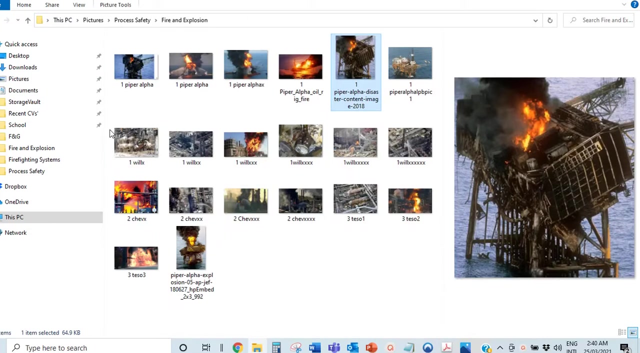 catastrophically and the pressure just bust out of the world seems like. you know, all this equipment, they are all welds, they are all welds around them and one of the seams got loose and fire erupted and that was it. so I think enough with the gory stuff. I think we can. we can do with those and just have. 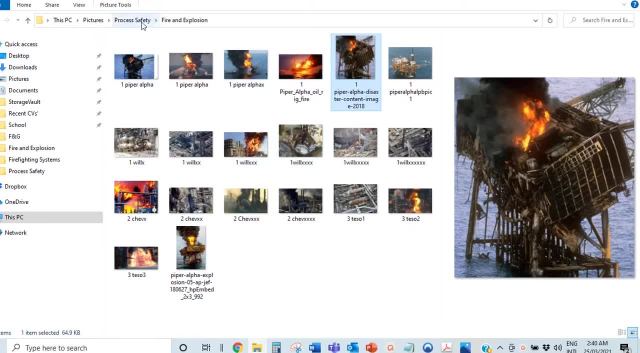 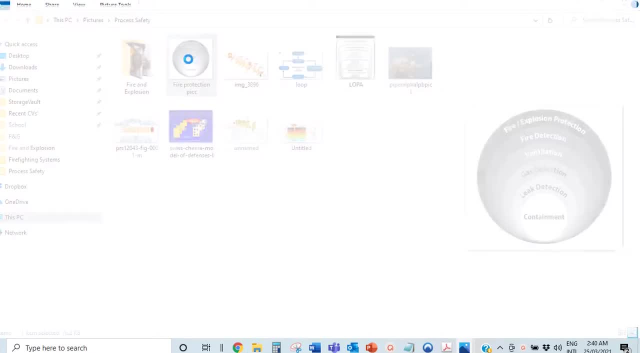 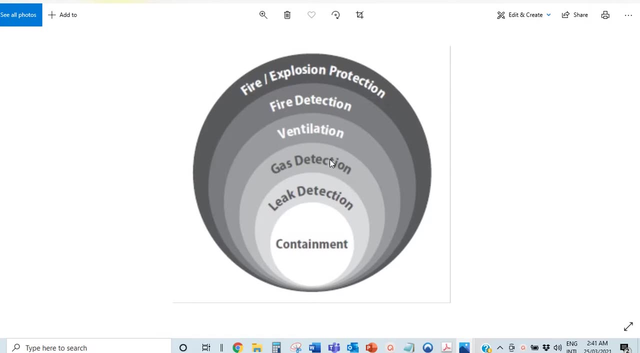 some peace from that. okay, so I want to talk about, like, what's process safety? so process safety- I think I would like to describe it with this drawing. it's kind of looked at as this study over at Tahoe great Wh. expand my own process safety research together with 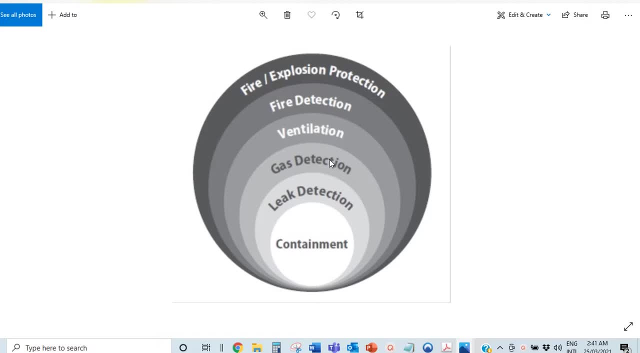 the clinical trials at faint and see what steps others came up with to show up with. so this is actually a technique for us where, if we start a계ng Joe incorrectly, dryiness and and then the downside begins to, so it's what it's. so the idea is preventing fires, preventing leaks that can cost 380, 00 to lots of people, like toxic gases or flammable gasses. so preventing fires and accidental chemical releases in chemical processes or facilities and when you are dealing with some very hazardous materials such as aurum gehen subjects as refi nghiere in refineries on aFe llegd in ref nghĩING eand train~. 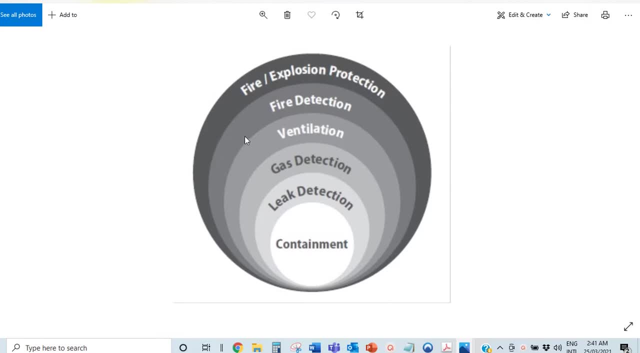 in oil and gas production. that is process safety, trying to avoid these fires or leaks that can lead to very, very catastrophic accidents, and it's different from health and safety. health and safety is mainly looking at the health of personnel and their safety. that stuff like wearing your hard hats, your helmets, your boots, your using your harness when you're walking from. 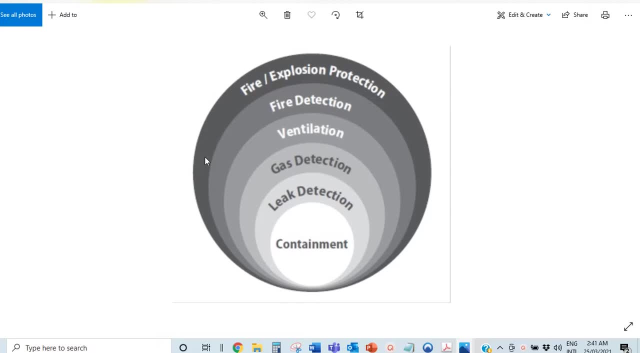 heights. that's it looks at act the actual person not designing the plans to be safe. so those are the main differences in process safety and occupational health and safety. so process safety generally refers to the prevention of unintentional releases of chemicals or very dangerous materials during the chemical process and this can have very serious effect on the 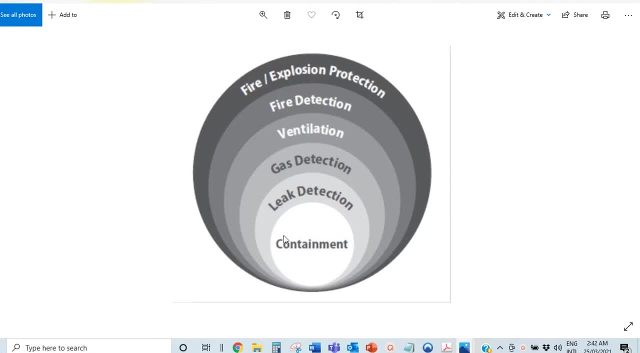 plants and on the environment. so this, this is the reason why we're talking about the process quality for these processes, because you is where we're going to start from, because you, you, if you've seen my other videos, you would see i talk, we talk. i i've talked a lot about has ups and stuff like that, so we are looking at. 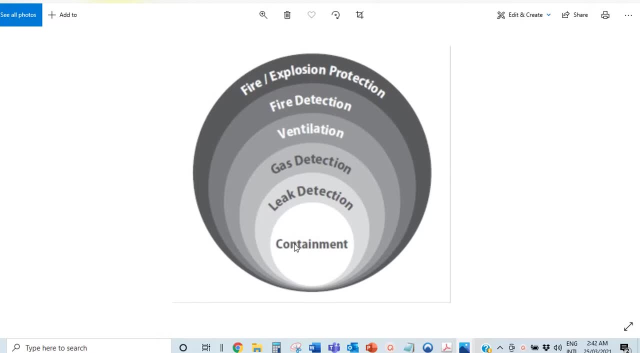 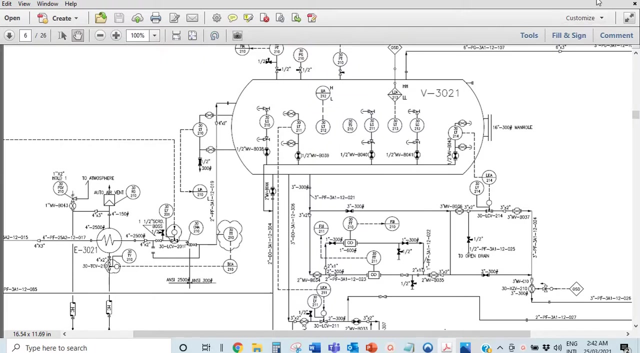 the very first thing is try to contain it. and how do you contain it? that means you have to have very good processes. your equipment are designed to standard the thickness, the material selection of all stuff like this, all your vessels on site, everything is on point. that is the first step. 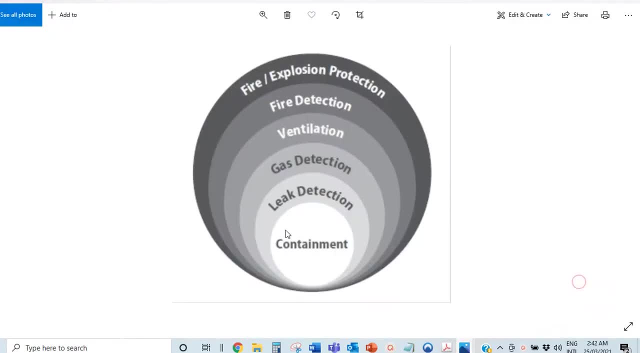 in this process safety thing to ensure that it is contained inside here, and that's why you have things like your, your loops, your, your alarms, your trips, to make sure everything is contained. we don't want any leak coming out. we want it to go from this vessel into the next vessel through the 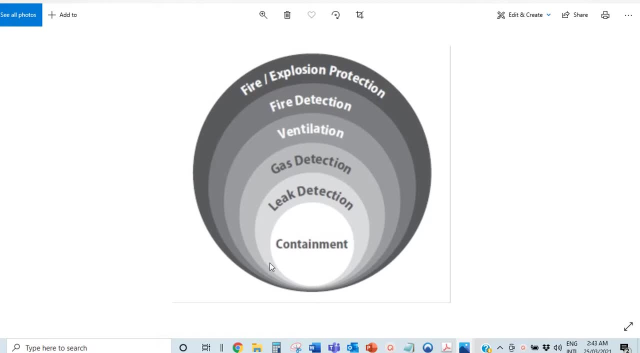 pipes through the pumps without any leaks. so what happens when there is a leak? that is, you we have, like a pipe alpha situation or the chevron refinery. what happens when there is a leak? it can be for a gas or for, or for a liquid or fluid, and then you should have leak detection. so what's? 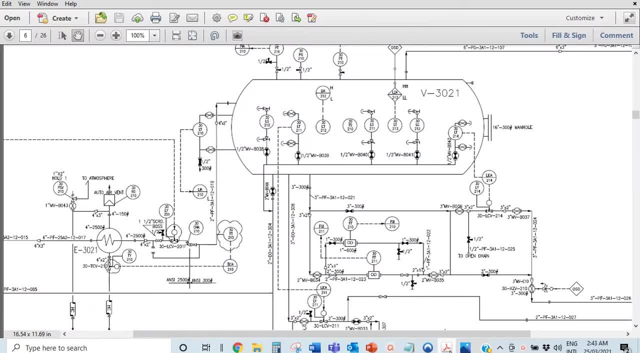 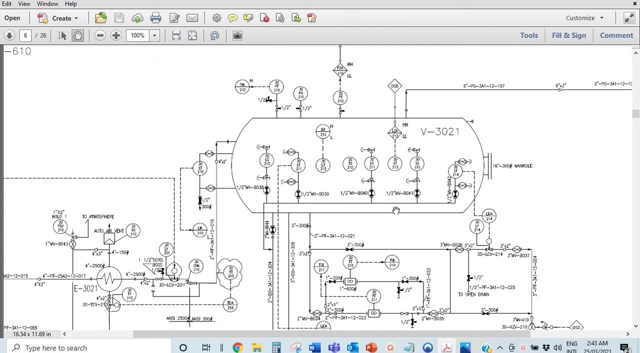 leak detection. leak detection is stuff like um your fire and gas detection system. so those are stuffs like um your your heats. i will do a video um explaining fire and gas detection, but that's mainly looking at stuff like your heat detectors, your flame detectors, your smoke detectors. that's what it's looking at. 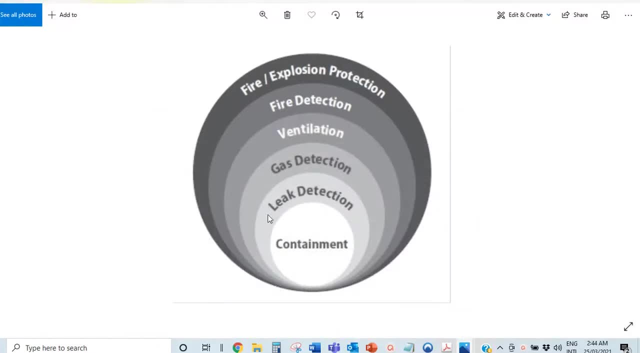 and if after that, if this is not enough, then you have gas detection. your gas detection is looking at stuff like gas when it escapes. so you have um, because this leak is the leak detection. it could be a fluid. if it's a fluid or a liquid like oil, not gas, then the only way you're gonna know is you're. 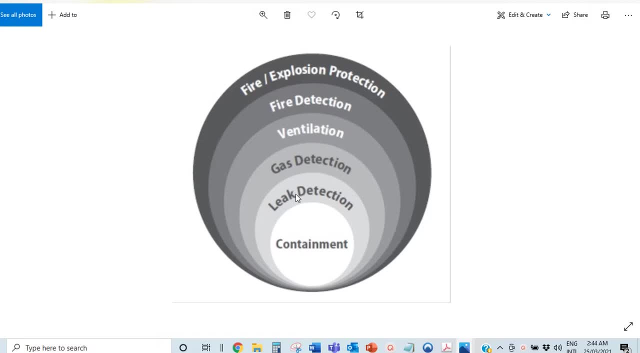 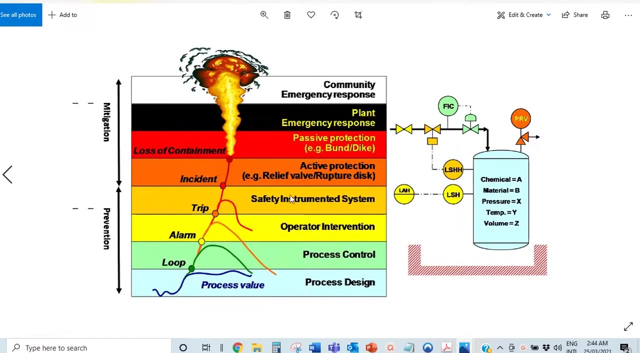 gonna have your your level trips which could lead to, um, your level alarms, which might alert the generator that there's something wrong going on, and then you have your level, your level trips which can kind of control it. so i have a picture here which kind of explains it. 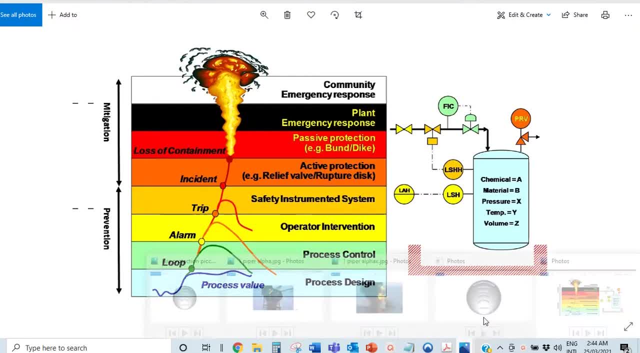 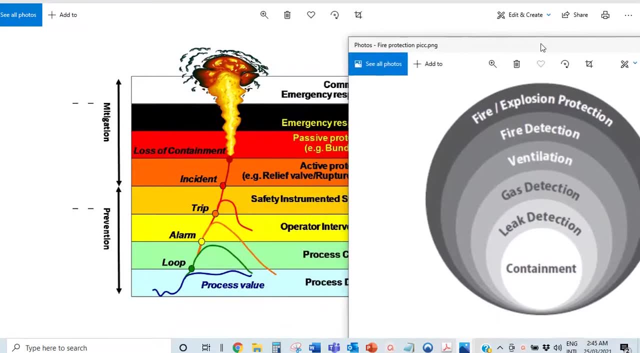 so i think i should put them both side by side. where's the other one? okay, that's this, so let's see what i can do with this. so, leak detection, that's your leak detection. um, so you have. you should also have a bond around wherever there's a lot of um. 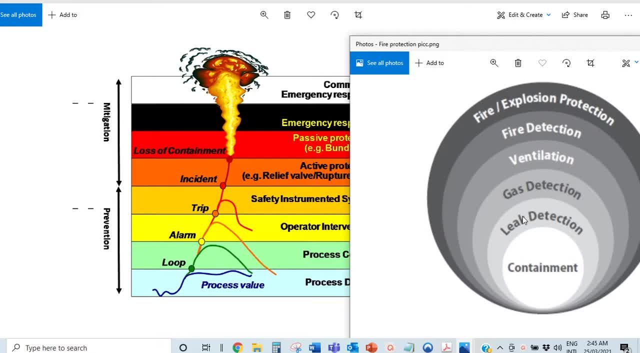 a leak, a lot of oil or liquid, hazardous liquid, there should be a bond to contain it. and then you have your leak detectors, your trips, your alarms that let you know, and of course you can actually see the stuff- who's in out. then there's your gas detection. you may not see the 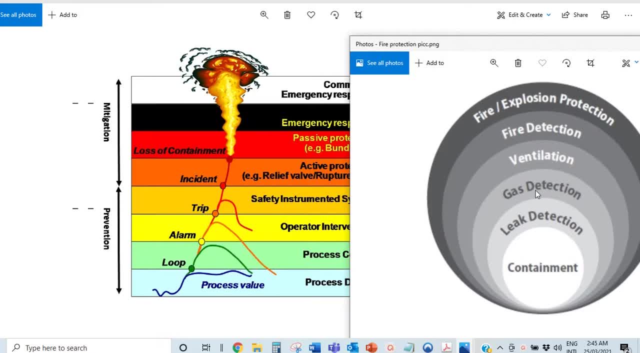 gas. depending on if the gas is colorless, you may not see it, but you would have specialized equipment like gas detectors, flammable gas detectors, toxic gas detectors, line of sights, gas detectors all around to make sure that if there is a leak, it detects it and there's an alarm goes off and then 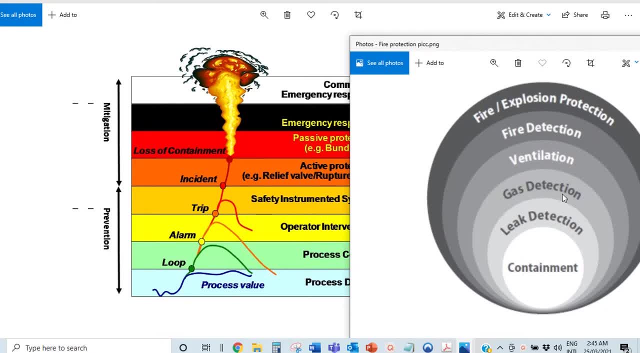 the plant shuts down and then, if this doesn't still catch whatever hazardous material has escaped. then there's ventilation. you should always think of separation distances giving, making the plants ventilated enough so that you don't have pockets of gases hiding around that could be ignited or when they emit an ignition. 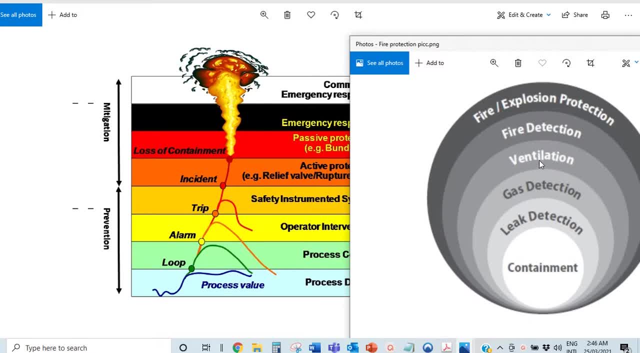 so you want to make sure it's properly ventilated so that the air can carry away whatever hazardous gas has leaked. and if then you get your, it hits an ignition source without dissipating, then you have your fire detection, which is your flame detectors, your heat detectors, and then, if those, if that. 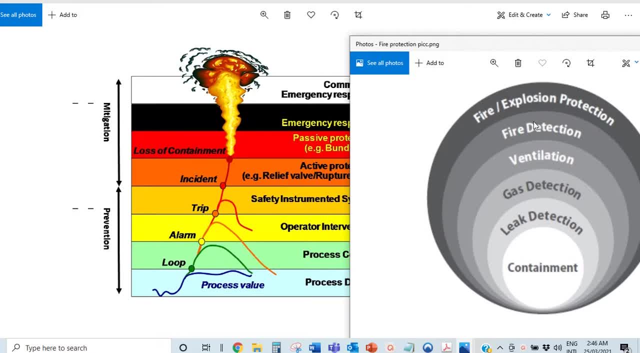 happens, the planet is shut down, and then you have your fire and explosion protection, which am it's mitigating factor. so, once this has happened, you are going to mitigate, you are trying to mitigate it from escalating up to this top position. all the way from here, you want to stop it from getting to. 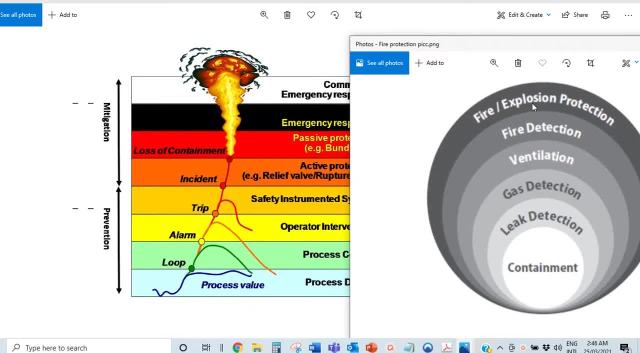 the fire and explosion part. and when this happens is when you have your fire and gas um, your firefighting systems, your hydrants, your monitors, your sprinklers, your gas suppression. that's when you start using all those. and when this doesn't work out well and the fire is raging on, then you 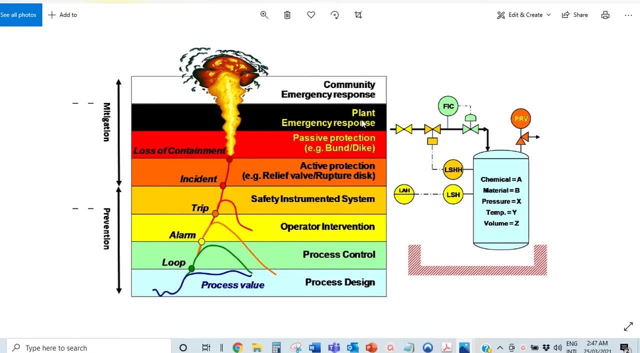 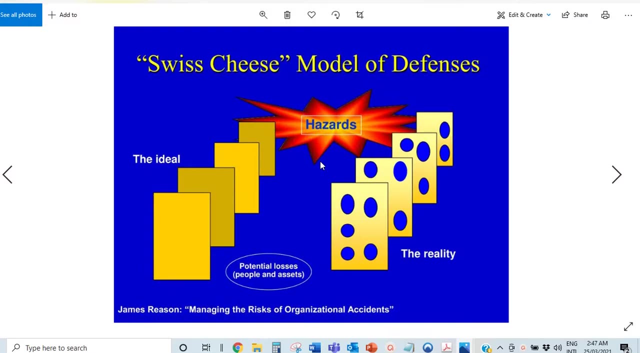 have stuff like emergency plants- uh, plants, emergency response, community emergency response. so i want to explain it with this also, or, before i go into this, let me. let me talk about what they call the swiss cheese model. so, um, this is kind of what, um, an idea of what, the swiss cheese model. 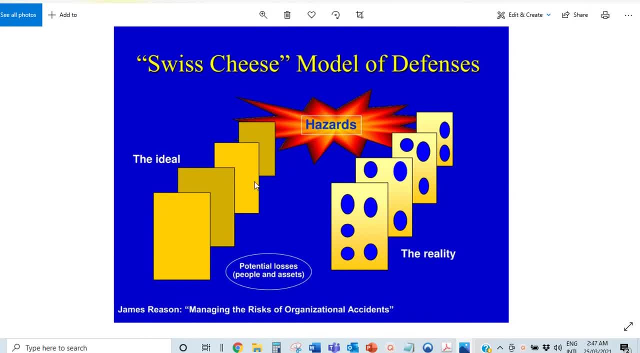 is it talks about, um it's a model of accidents, um, like prevention, that illustrates. it kind of explains um the layers of defense that lie between the hazard and the accidents and how each layer is flawed. so let's say this is one layer. okay, i think i should. 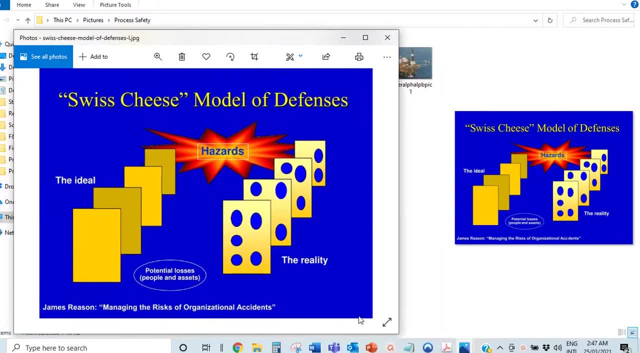 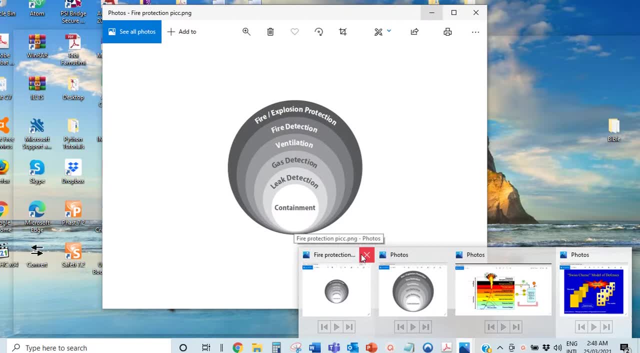 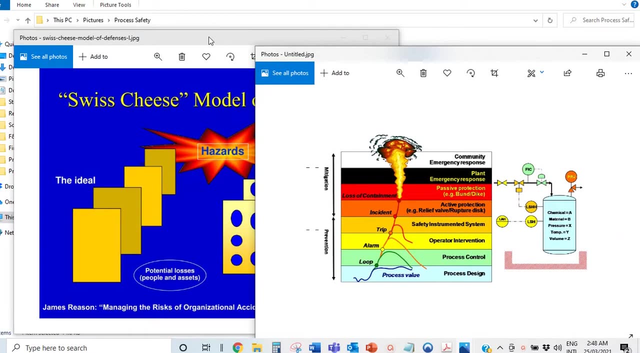 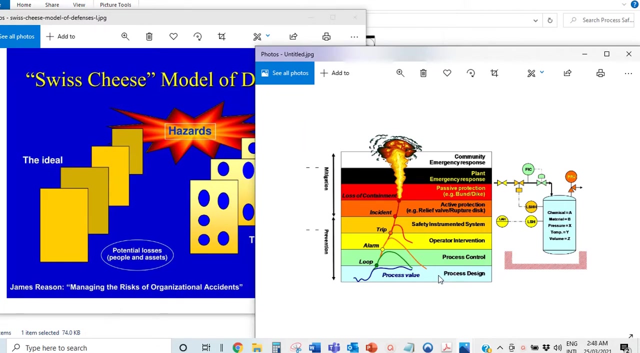 pull this to the side also and pull up- uh, what's it called? let me get rid of this- gory pictures and then okay, so the swiss cheese model. so each this is a layer process design, meaning the first thing you have to do is design your plants safely, which is like saying inherent safety. that means you should have. 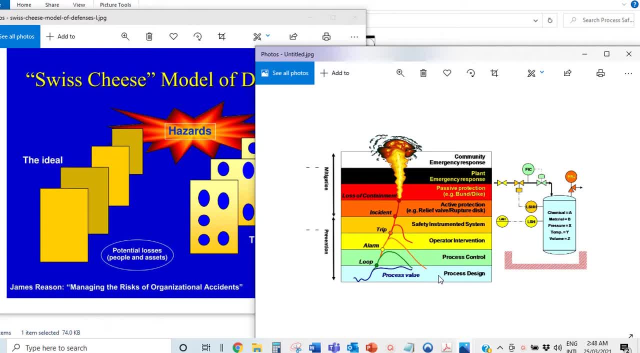 safety built in from scratch from the very beginning of the design process so that it is inherently safe. the the whole plant is more or less- um, should i say- aware that an accident can happen and it's trying to prevent it every step of the way. that an accident tried, or 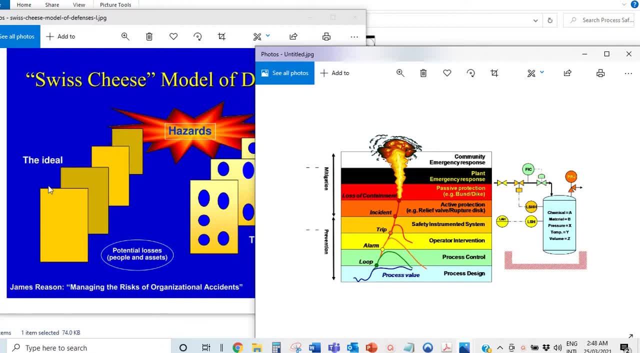 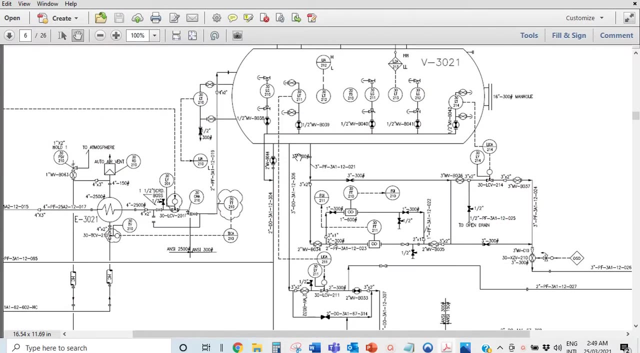 tries to occur, it prevents it. so that's process design. you can look at process design as your first barrier here. you can look at process control as another barrier here. so that means your loop. that is stuff like this here, where your loop, which your loop, is like: okay, this is a vessel operating. 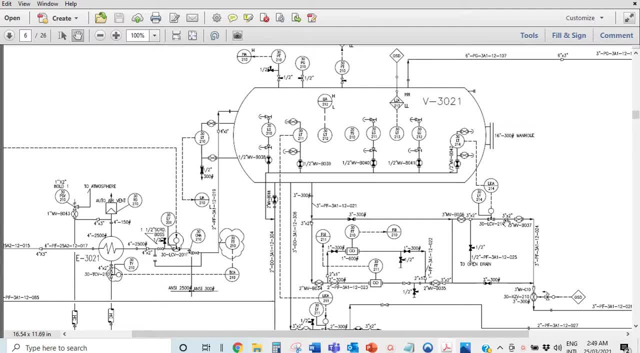 if the vessel gets too full, your level transmitter automatically opens this valve. the liquid flows out from here, so the level drops, so that you don't have spill or liquid carry over. and if the if the it's still getting full, if this cannot handle it, it would. 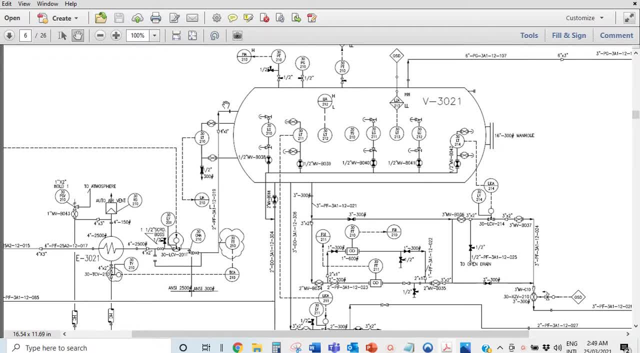 automatically close the inlet so that there is no flow into the vessel. that is the idea. that's kind of like what a process loop is about. it is sensing the temperature, it's sensing the pressure, it's sensing everything happening in there and it's sensing the pressure. it's sensing the pressure. it's. 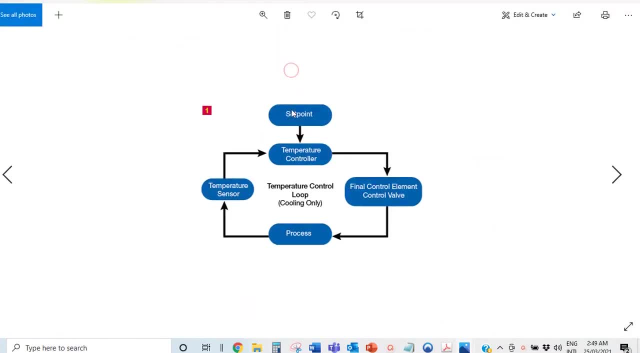 automatically, automatically responding. so this is like a picture of um, like a loop. it's just a very, very basic picture. so let's, this is all about temperature. so there's a temperature controller and it has a set point. when that set point is um, when it hits that set point, let's say the normal. 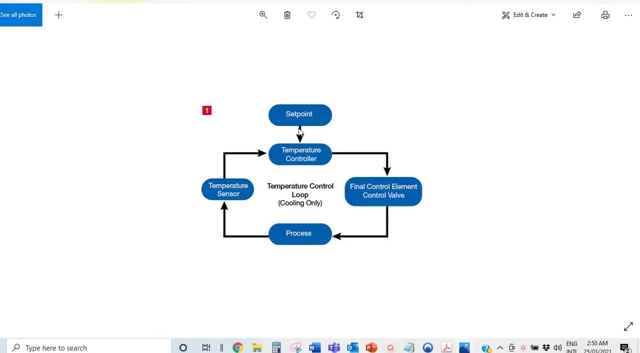 operating is 50 degrees centigrade, it hits 70 degrees centigrade, the set point might be 90 degrees. after that set point maybe the next thing is: um is an explosion, or it's going to explode, or it gets too hot, then it's automatically. the temperature controller tells the control valve. 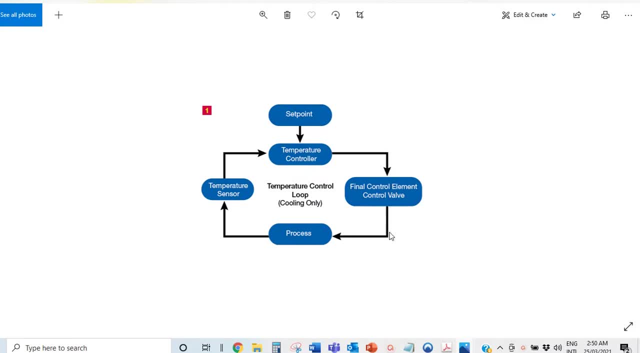 the final element in the control valve that you should close now because the heat is getting too much, and which automatically cools down this process, and the process is continues running, continues running till if the temperature starts getting high, the sensor picks it up. it tells the controller. the controller hits the set point- this is now too high, it tells the valve. 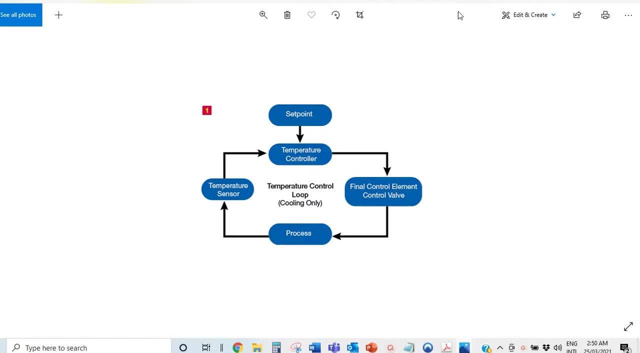 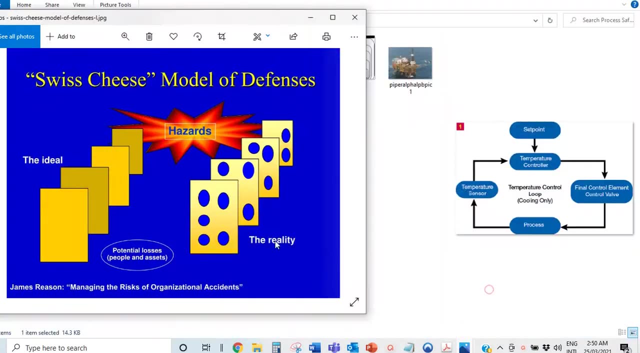 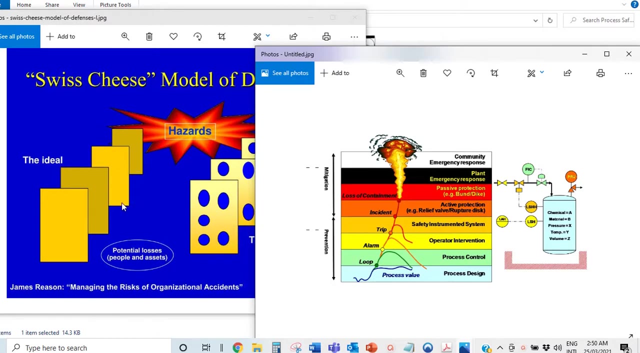 to go close the inlet of wherever the heat is coming from and like that. so this is a very basic form of a loop and um, so your loop can be another, another barrier, and then you have your alarm. your alarm needs an operator intervention. so that means when an alarm goes, an alarm doesn't do anything. 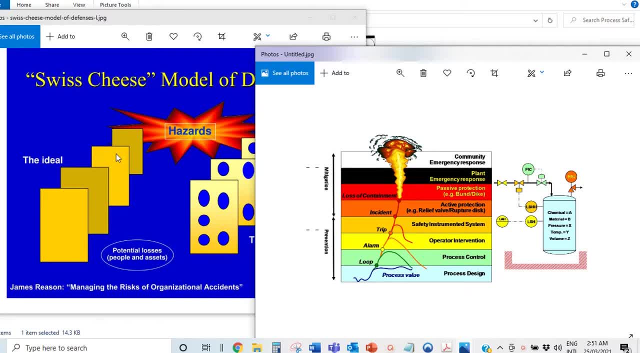 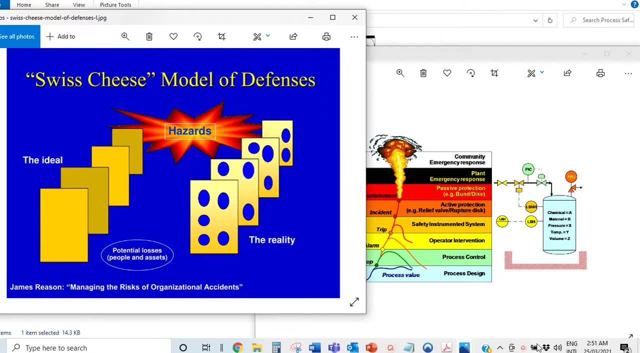 specifically or don't tell the people, other than tell the people that there's something wrong happening. so the thing is why this is used a lot is because when we design well, everyone looks at it like I've done a fantastic job. the design is top-notch design. but no matter how top-notch the design is and foolproof it is, 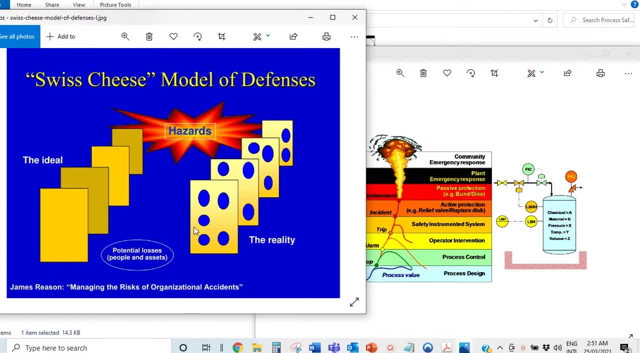 even just um like talk of the Chernobyl accident. no matter how foolproof it is, it has some holes. it definitely has some holes. either the operator was not trained well or maybe when there's a power failure for one second, something messes up in the system. there's something. it cannot be 100 perfect, so these are. 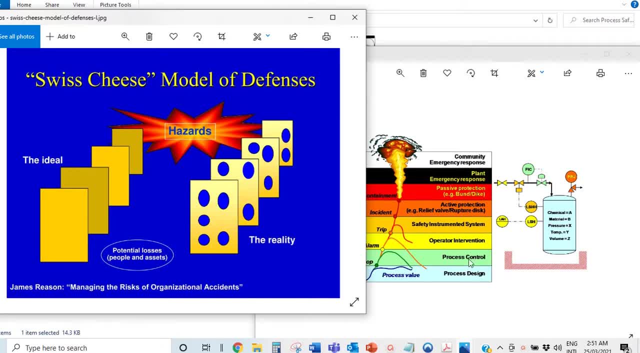 the holes in that system. and this is the next barrier: process control. there are holes in it here. this is so. they are saying this is the ideal, but this is the reality. every system, every barrier or safety system has some loopholes in it. that's so. but the thing about process safety is: we want 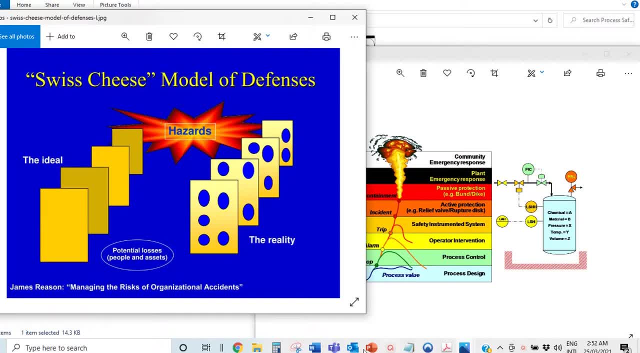 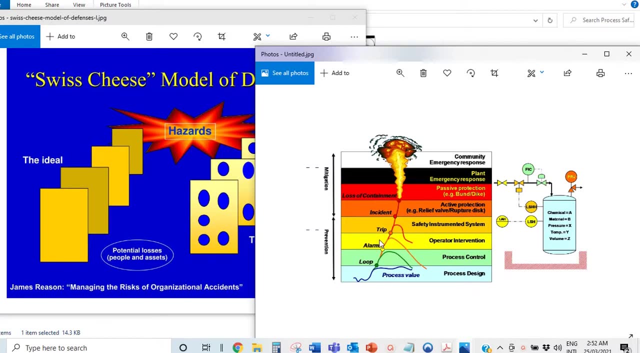 to stack enough barriers all the way around, um like we could have up to 10, 15 barriers. so, starting from designing it well, to controlling the process well, to setting an alarm so that, and if the operator doesn't work up, answer that alarm and quickly do what it's supposed to do, then there's a trip which should happen automatically. 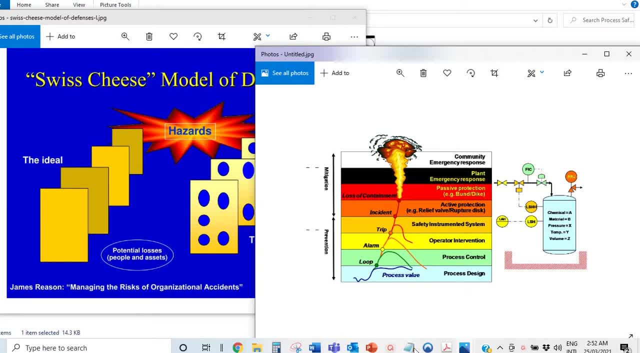 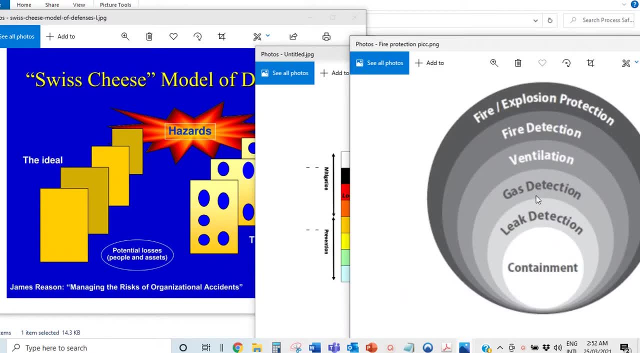 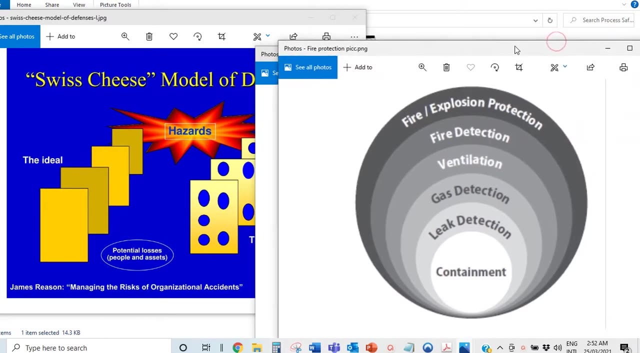 and if that trip fails, you now have the leak. if that leak, that leak to um, you have your leak. and if that leak is not detected, then there's still ventilation to help it dissipates, and if that doesn't happen, then there's fire. so there are plenty, a lot of barriers in place to make sure that we don't reach the top. 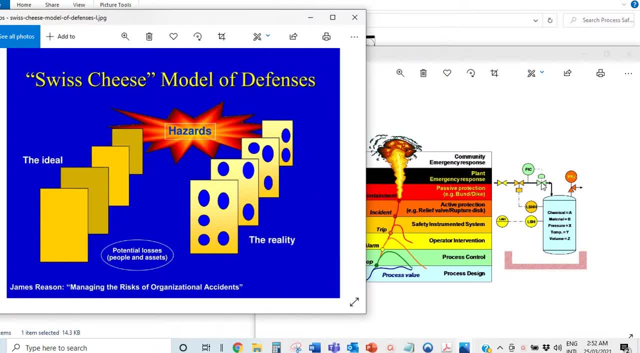 event which is like a nasty fire and explosion. so so when um this, the so the theory is actually like is looking at several slices of cheese all stacked on top of themselves, that's all this sizes of cheese snacks stacked on top of themselves. and the idea is, if 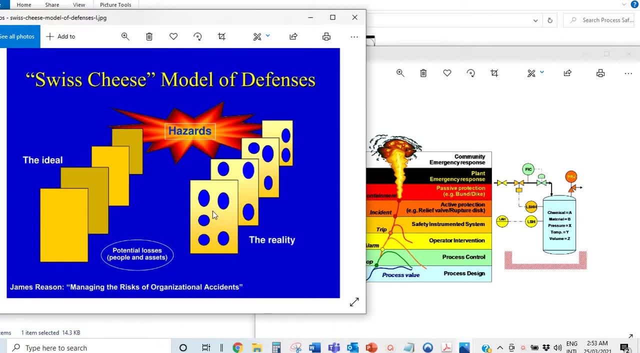 the holes do not align, then a beam of light cannot pass through. and if a beam of light cannot pass through, that means there's one of them has blocked it. one of these barriers has blocked the lights. the light is the accident. if it doesn't pass through, then we are safe. but if somehow, or the 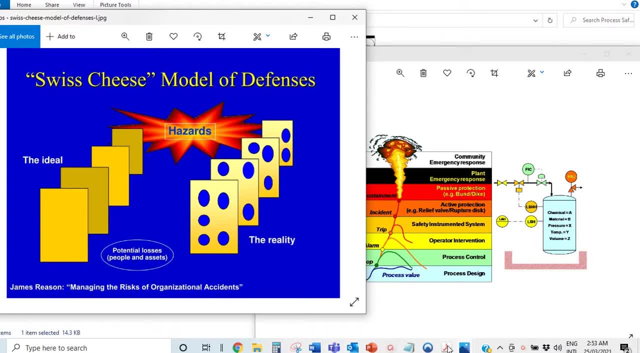 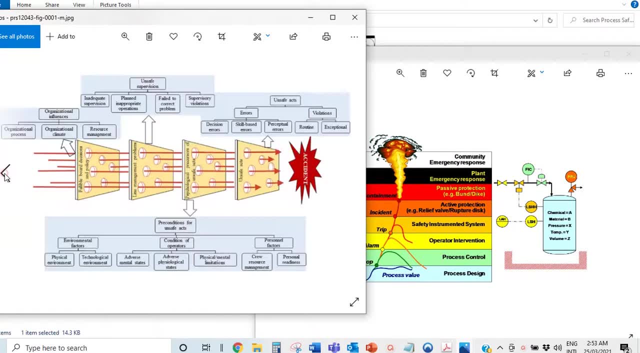 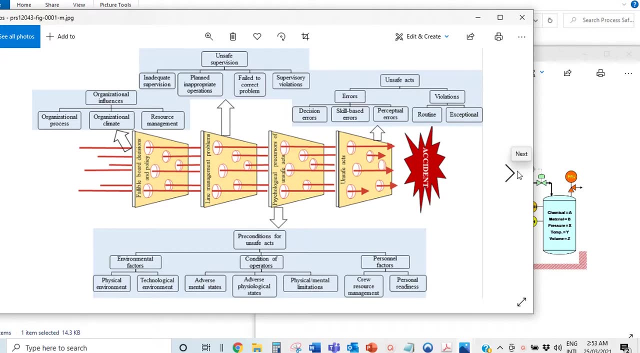 other. they all line up, then there's going to be like an accident. so that's what the idea is all about and that's um I want to look at. I think I have, yes, so this is something we can look at. looking at the cheese um, the Swiss cheese model. so you have. 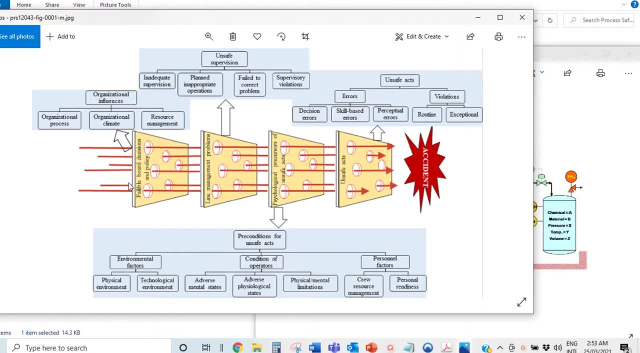 um, your, your, these are different. um, there's line management problems, psychological precursors of unsafe acts, on safe acts, and when they all line up is when you have an accident. but you have so many things that can lead to an accident and it happens, happen every day. it could be the operator is sleepy, it could be um his the operator is sad. it. 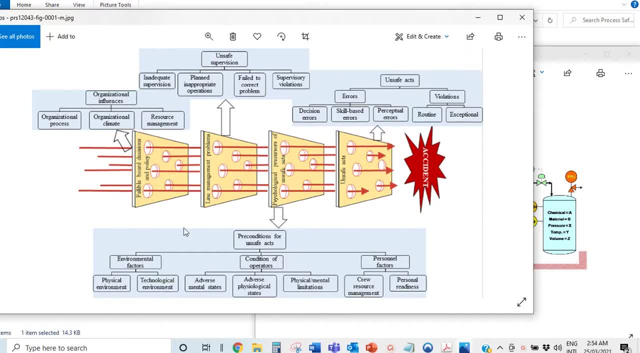 could be. the system has a flaw, not designed perfectly. it could be environmental factors. that's like wind. you never knew that there could be a hurricane which pulls out a pipe, or you understand, there's so many things that could lead. make all these holes align on that's. 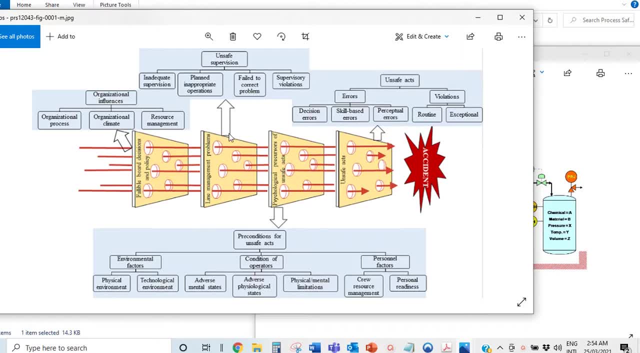 a very unfaithful, just like as I described in pipe offer. some guys were working on um pump a. they finished their shifts. they didn't do a proper handover they would. they probably thought that everyone would know that this pump was not supposed to be turned on and they went, and they went home. 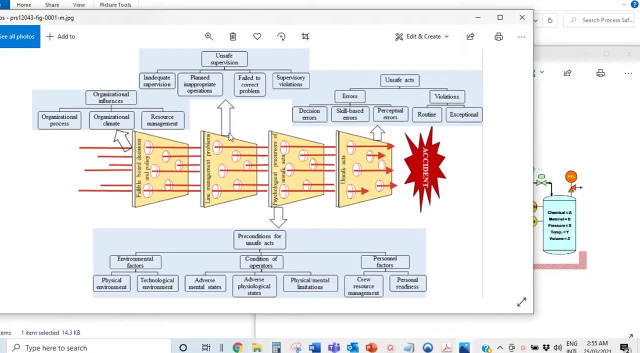 and the new guys who took over didn't know that that pump, so that was a gap, that was a hole and they tried turning it on and that's and that. but there should be procedures, place, like your permits to work, which should let you know that once if i can't finish this job, i 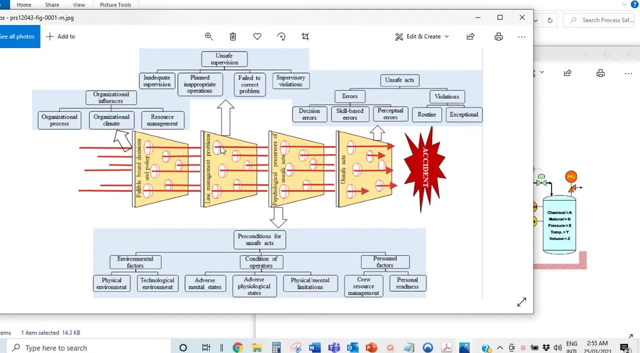 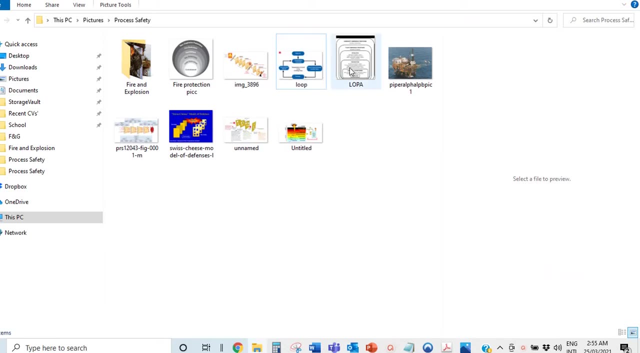 should allow my supervisor, or the allowed the supervisor of the next shift, to know everything that's happening, the present state of the of the facility. so there's so many things that could make everything align, and once everything aligns, then you have the the problem. so this is also. 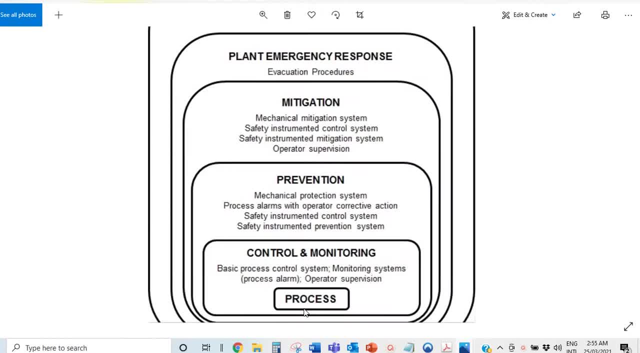 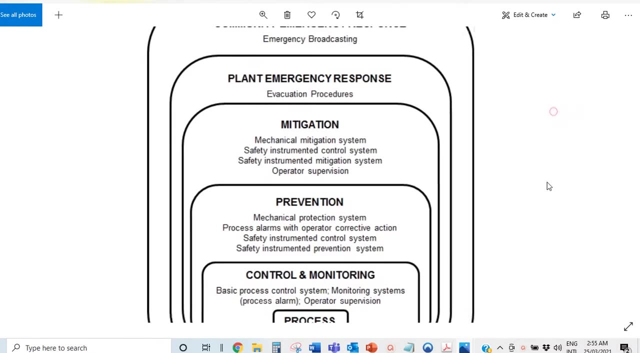 another way of looking at it. you have your process, which is your um. your start doing stuff like us, up at every stage. they are documented. there's documentation to make sure that we don't- things do not um escalate and get out of hand. so you have your process, which is done. 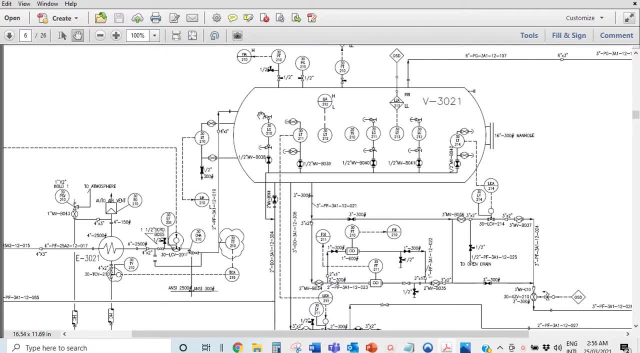 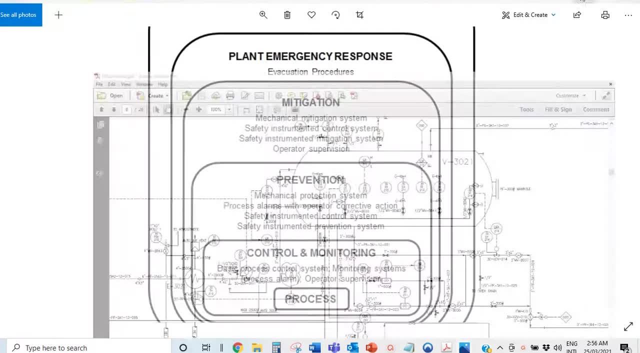 this way. this is a p and id, but you do your has up or needs. you do so many studies on it to make sure that your PR and IDs are good. there's a lot of review that goes into it. and then there's your control and monitoring, your basic process control system, monitoring system. those are your 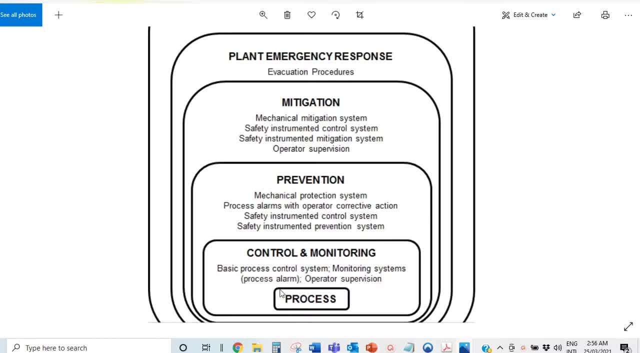 trips, those are your alarms, those are your operator supervision. so many things go into the controlling and monitoring. that is after designing it to be foolproof. you now have your control and monitoring system, which are people, the systems you've installed now. if those fail, you now have. 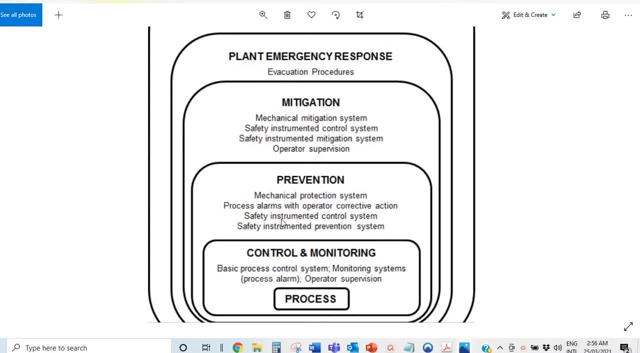 your corrective action. you have stuff like your CIS safety instrumented systems. those are very, very highly reliable systems that fail maybe one in 10,000 times. so they are very expensive and they operate stuff like your valves, your trips, those. those are there to make sure that, even if 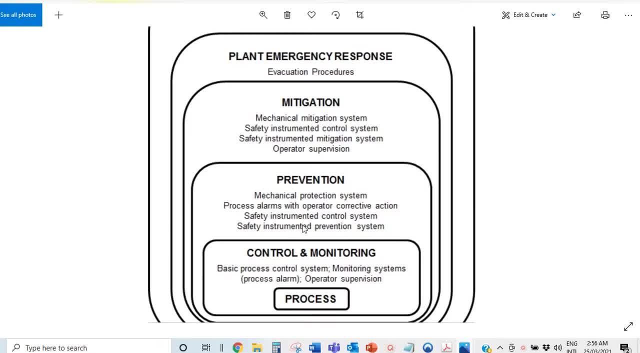 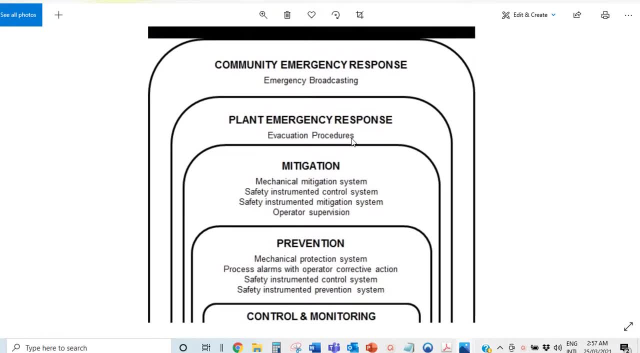 everything fails, they would automatically kick in. and even if it fails, you now have your mitigation systems. and then you have your plant immobility emergency response, which is okay, and the alarm for the whole facility is ringing. you have, you have your. everyone runs out to the master points. you have your emergency response from, from. 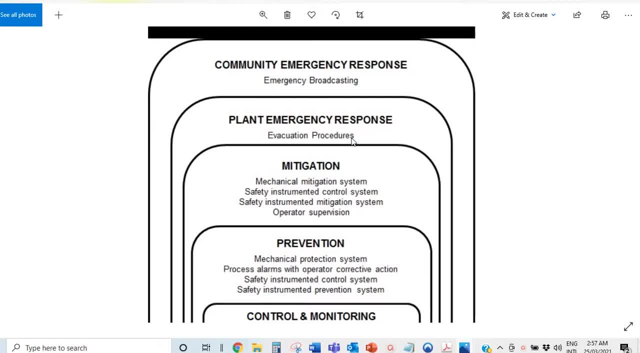 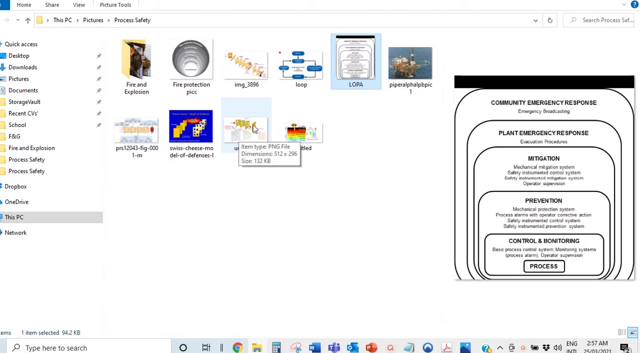 whatever town you're close to your ambulance com everywhere, everyone shows up their fire response everybody. and then you have your community emergency response. everyone in the communities are lot that there's something hazardous going on. so that is more or less in a nutshell. what process safety is about is trying to make sure that whatever scenario we have that could get very 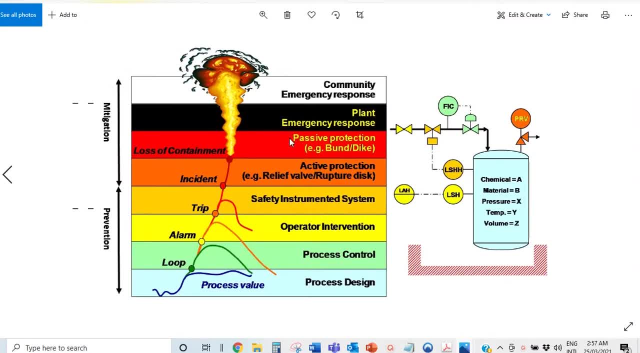 very nasty. we have a situation in place to prevent it to, to stop it from escalating to a full-blown fire, to a full-blown fire, explosion and stuff. so this part is the prevention, which is kind of what i explained also in my bowtie video. you can see this is the process here. this everything is blue. 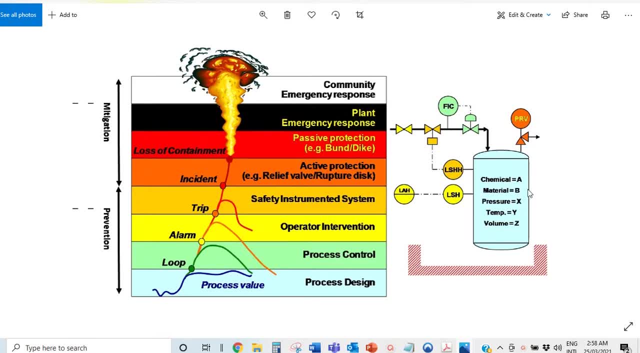 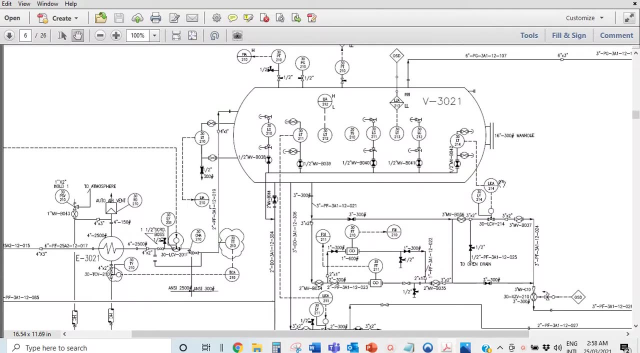 you are in the process, design, process control, everything is working normally. then there's a problem: um, an alarm goes off. also, it's very, very important to do your alarm rationalization, which means because when you even look at this drawing, there's so many, so many alarms everywhere. there's your temperature alarm, your level alarm. 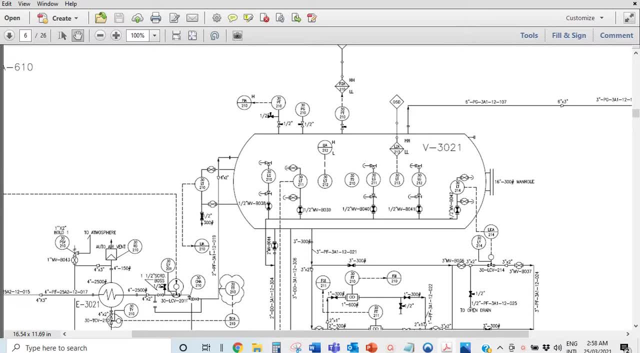 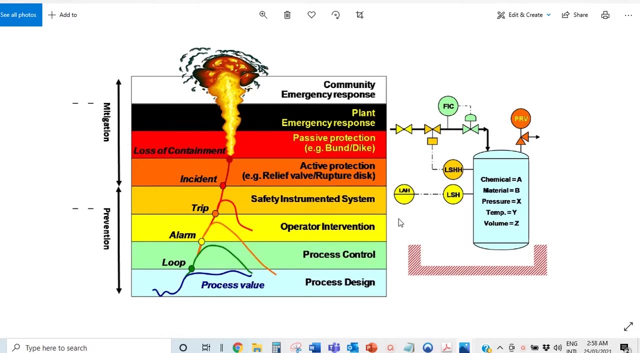 your pressure alarm for just this vessel and they are like 20 vessels in a small facility, dockless of facilities with hundreds of vessels. so you that alarm what happens? you want to make sure that you are rationalize the alarm. you don't want an alarm that doesn't is not really a critical. 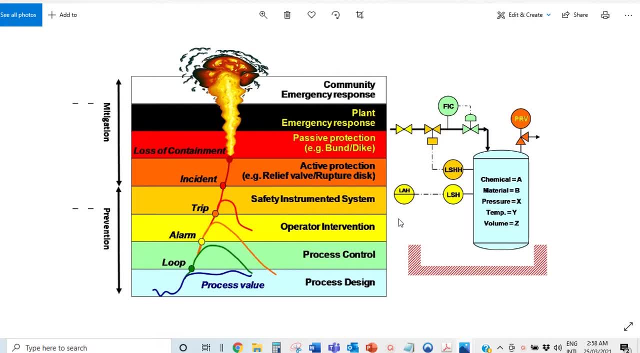 alarm just sounding and blaring all over the place. you want to set the alarms in a way that they everyone understands how, um should i say how important or critical each alarm is based on the sound, the lights that comes um, the the flashing lights. so, firstly, all alarms. 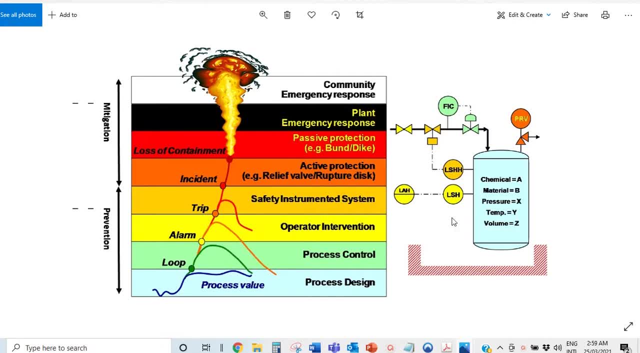 should be properly tagged so you know where the issue is coming from. if it's from vessel a, if it's from vessel b, then, um, it should be described: if this is a low alarm, if it's a high alarm, if it's a, you understand then the um, the set points, everything is set up in a way that it's. 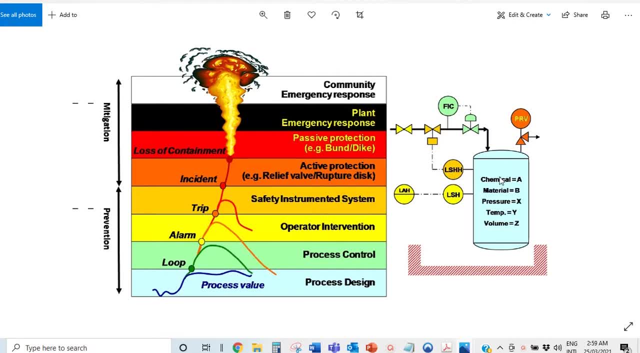 should know the set points, like: okay, this alarm goes off when it's 50 degrees centigrade. it should all be clearly written out in a, in a book that the operator has is very, very easily accessible to the operator. then you have your level alarms. you use the alarms. you should know the set points. 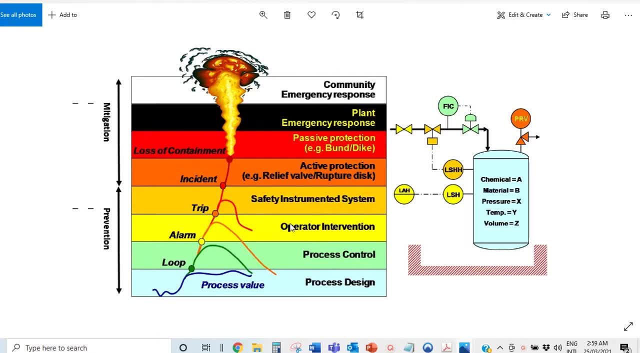 so that if you know that if this alarm is sounding, maybe you've hit 50 bar, if this alarm is sounding, you've hit 150 degrees centigrade, which are not supposed to hit and you should reach and you should have the potential causes. why is this happening? that would tell him how to solve it. 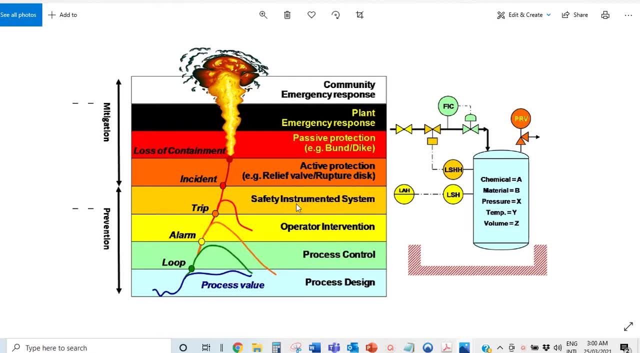 and also it should show the consequence of inaction. so if there is no action, what happens with this alarm? if there's no action, what? what's the worst case scenario? and then it should also tell the operator what he should do, so he knows what to do and he knows what happens if he doesn't. 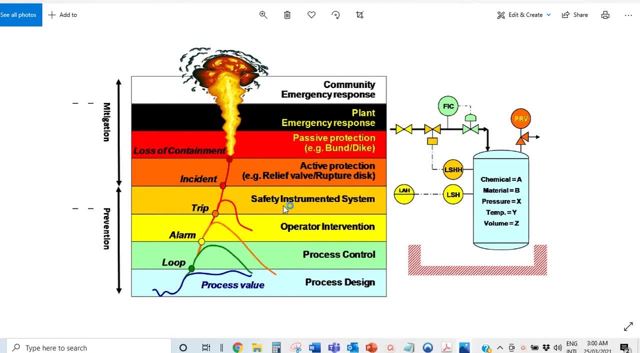 do it and then um how much time he has- if he has um one minute, if he has two minutes- before it escalates into something else. you know you should rationalize the alarms and class them, because that deals with somebody actually acting, doing something to prevent it's rising to the next stage. 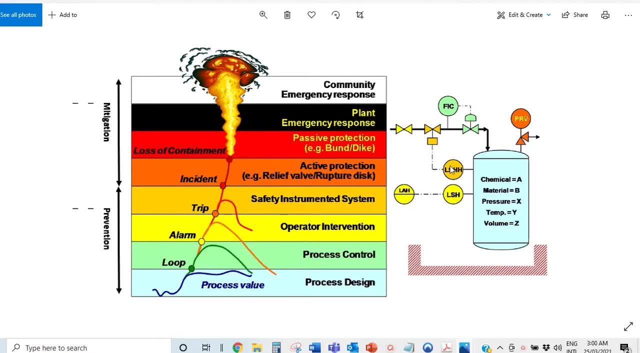 then you have your safety instrumented systems, which are your trips. which is this your trips? uh, is what closes it? um, the vessel. let's say the vessel is getting to full and the operator doesn't do anything with the alarm. the trip would tell him that wow. 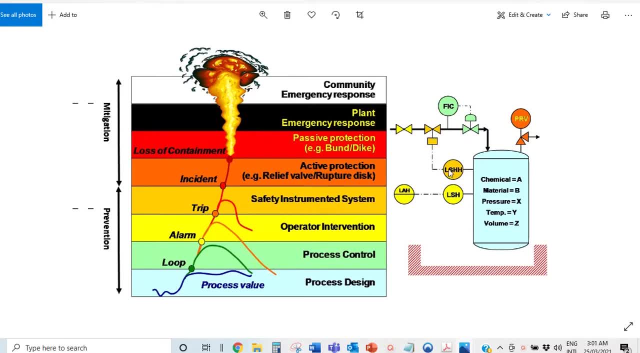 the trip would automatically close without the operator doing anything. but you don't want to shut down, right? no one wants to shut down, so it's better the operator does something and puts the process back in control. before this, before the the this um vessel is shut down, and then, if it's, 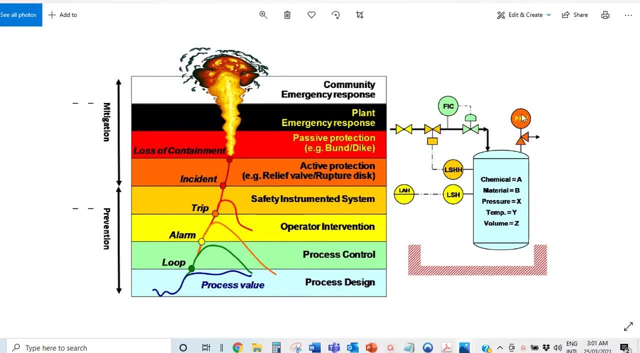 not shut down. of course you have stuff. if it's a gas, your peer, your prvs or psvs will pop and relieve to the flare, and if it's it doesn't pop, then we're in trouble. this could actually rupture and you have a rupture and then that's lots of contaminants. if it's heats, um. 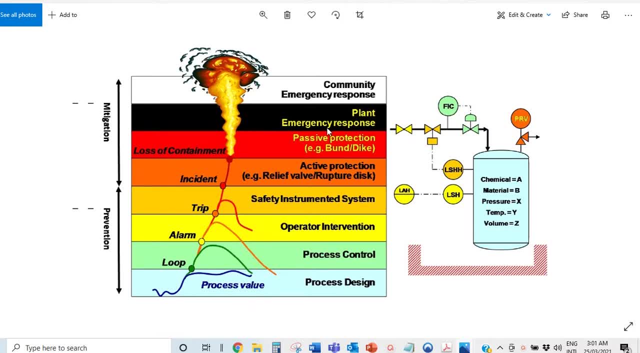 catches an ignition source, there's a fire, and it's not everything that is fire, something they deal with very, very um. some plants deal with very toxic, um chemicals that once you inhale them, there's. there was an accident, i don't know, maybe, maybe about what, like 50, 60 years ago. i can't remember the name. i should do some research. 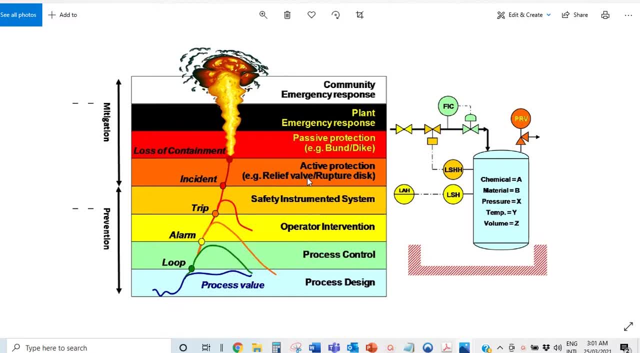 that it poisoned almost the whole town, the water supply, you know that kind of those kind of accidents. so that's what process safety is all about. i think i've been able to explain to a reasonable extent and, um yeah, thank you everyone for watching. my name is sharon toby. this is 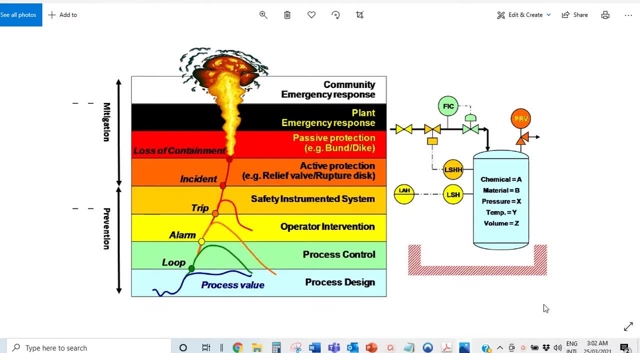 promoting safety engineering. please like my video. thank you and subscribe to the channel. have a lovely day, thank you.